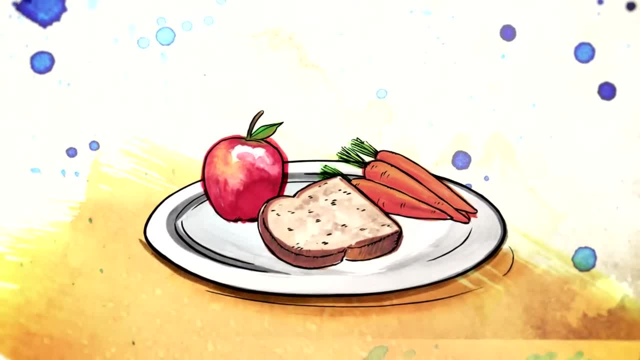 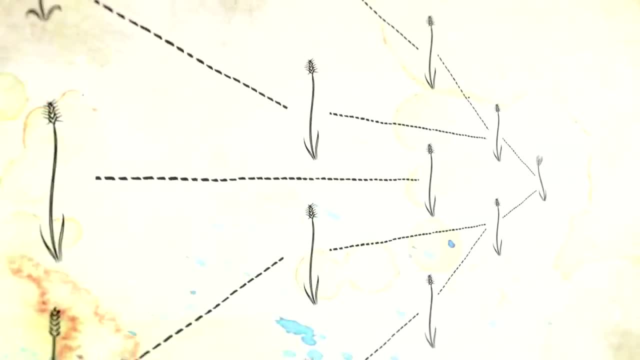 vegetable and grain that ends up on your plate tells a part of the story of our relationship with, and development of, food-producing plants. For example, wheat is the product of a cross between three different grass species, which is reputed to have happened about 10,000 years ago. Our 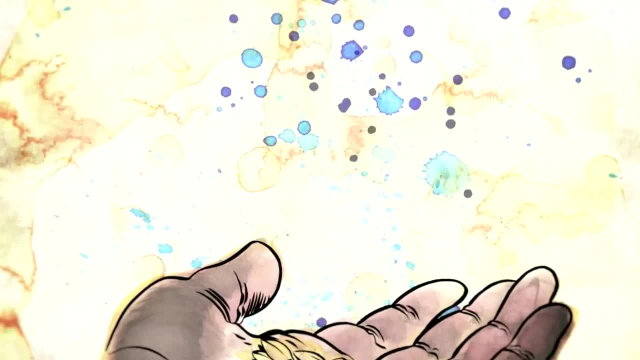 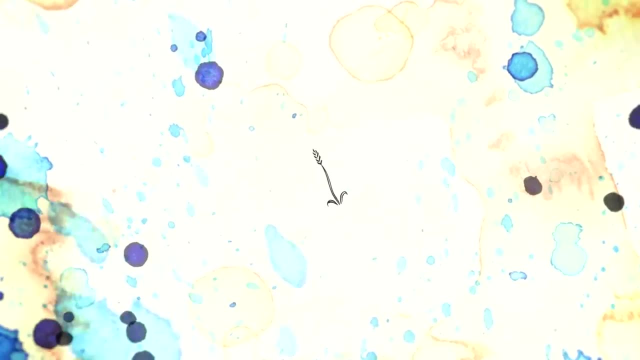 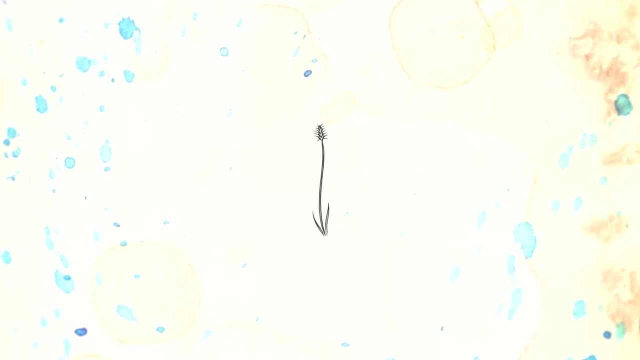 ancestors simply saved the seeds of the plants with desired traits for planting the next year, but the process of selectively adapting wild plants, also known as domestication, was quite slow. In order to speed up the process, farmers and scientists over the past 300 years have been cross-breeding plants of the same species. 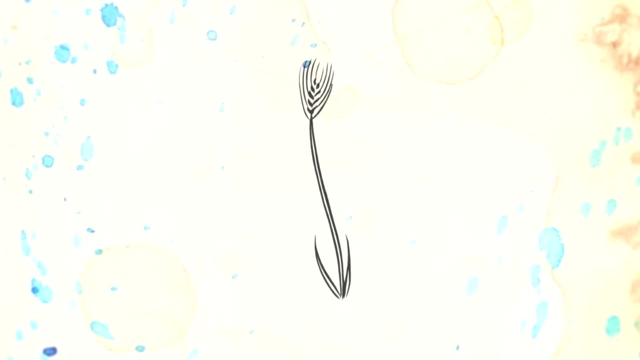 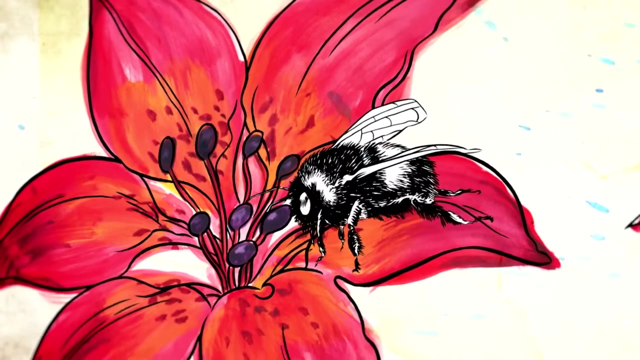 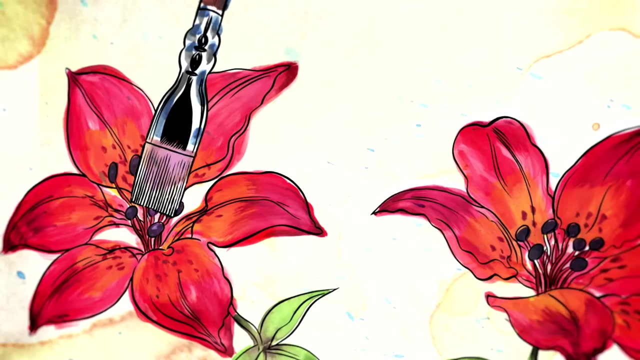 altering their genetic expression and creating new desirable traits in a much shorter time period. Cross-breeding of plants occurs through cross-pollination, a process where two sexually compatible plants happen to cross by virtue of pollen being naturally carried by wind or insects. More directly, plant breeders deliberately select and cross-pollinate the 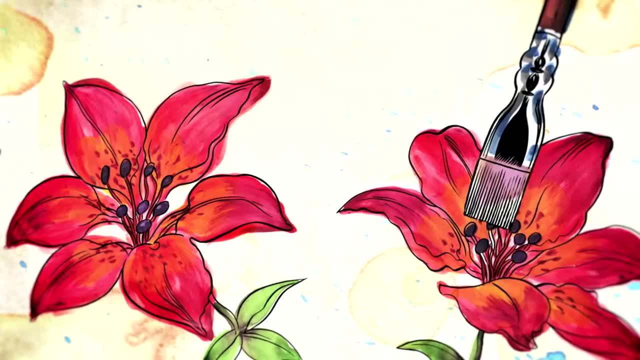 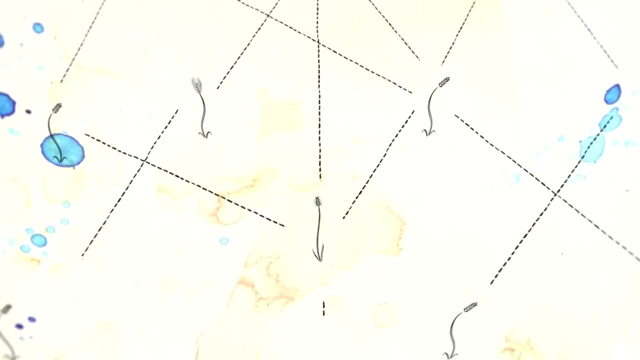 parent plants for their specific traits, transferring the pollen from one plant to the epistolate of the other plant. In this way, they develop a plant that may rarely occur in nature and one which has outstanding attributes of both parents. However, the development of 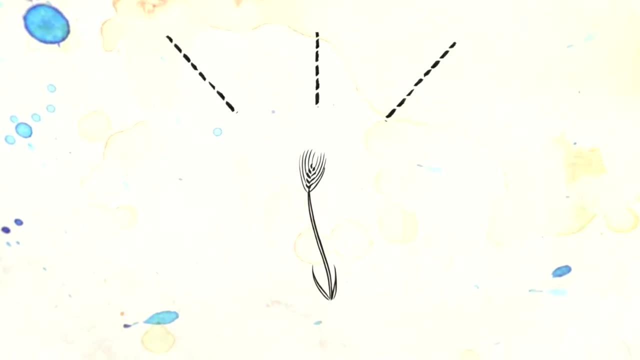 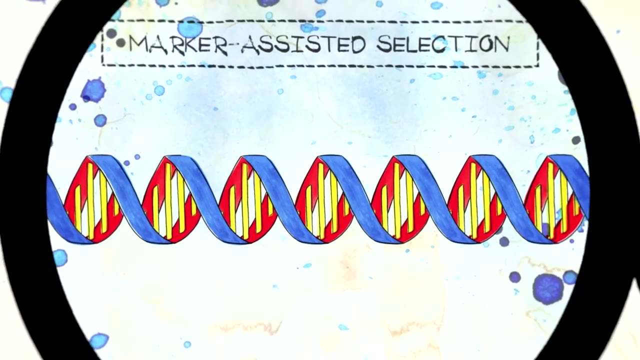 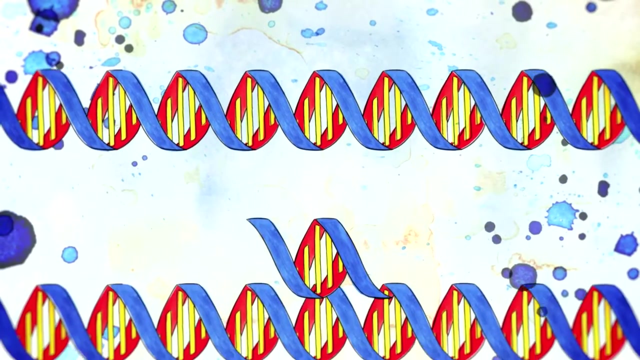 reliable new varieties through traditional breeding takes many years, if not decades. Today, cross-breeding uses molecular biology tools, called marker-assisted selection, to help guide and speed up the process of selecting the best parents and traits. Genetic engineering means copying a piece of genetic material from one organism and 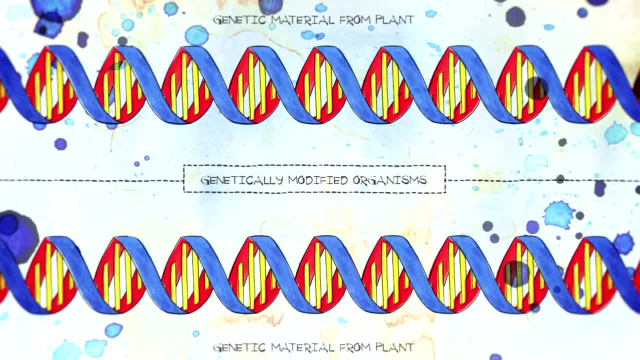 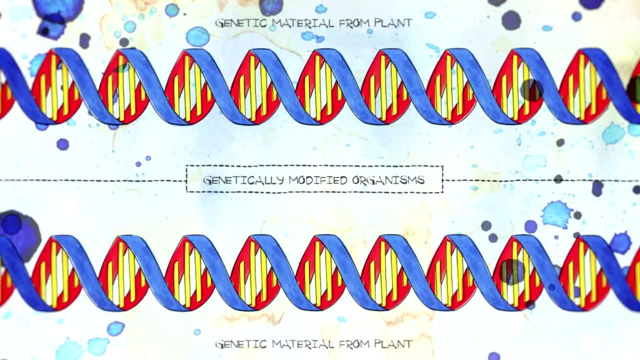 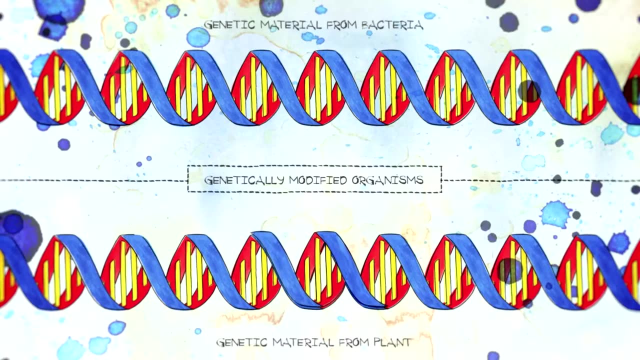 using it in another. Genetically engineered plants are called GMOs or genetically modified organisms. While many GMOs involve the crossing of genetic material of plants solely within the same species or genus, other GMO plants contain genetic material from bacteria that provides resistance to pests or herbicides. Crops commonly modified using this technology. 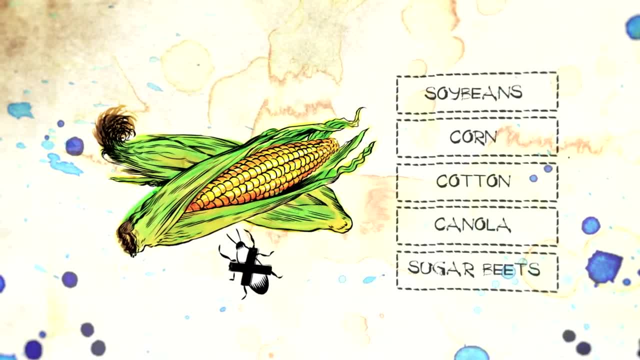 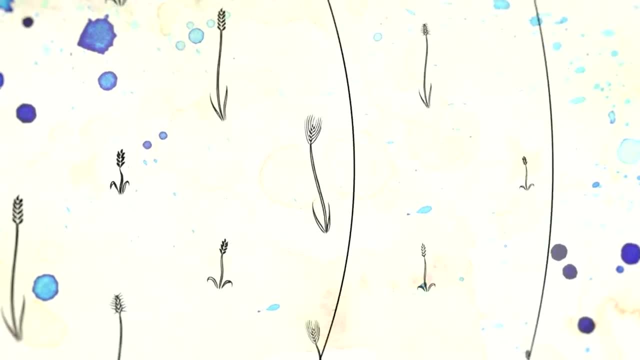 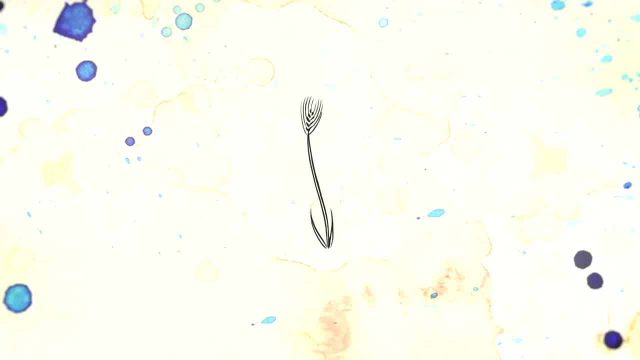 include soybeans, corn, cotton canola and sugar beets. Another method of plant breeding over a short time frame is to expose the seeds to chemical or radiation treatment. This is called mutagenesis and can result in altered and potentially beneficial new plant traits that would be further selected and developed. The value of food cannot be.